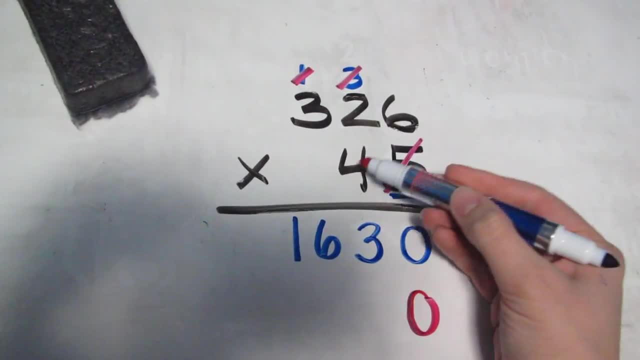 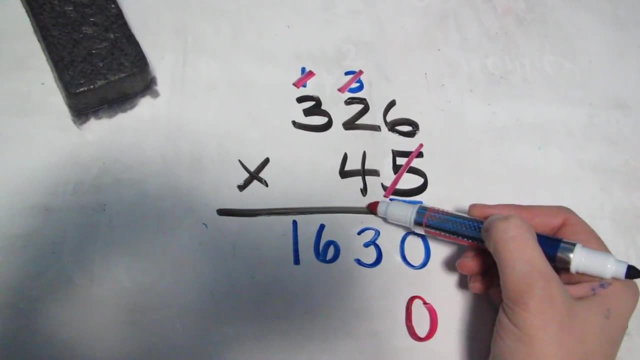 I'm not working with the ones anymore, I'm working with the tens. That's where the 4 comes in. So now we're doing 326 times 40, because the 4 is in the tens place. So here we go with this. 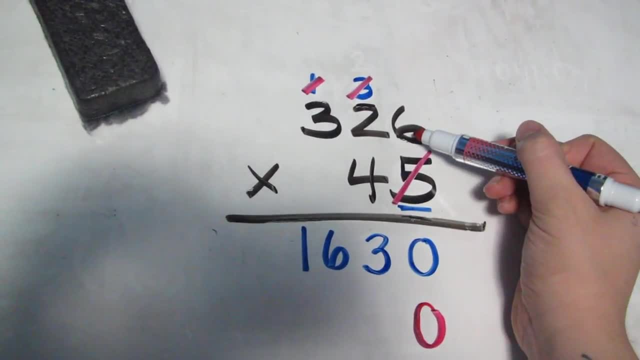 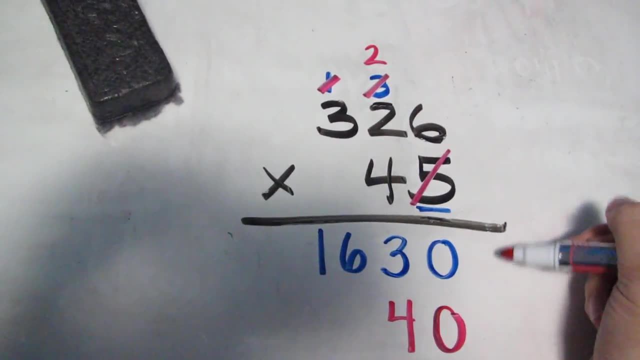 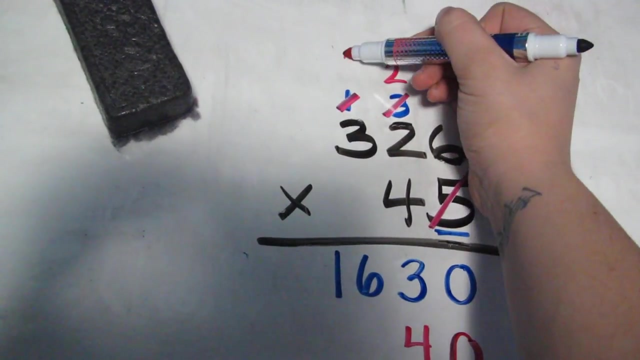 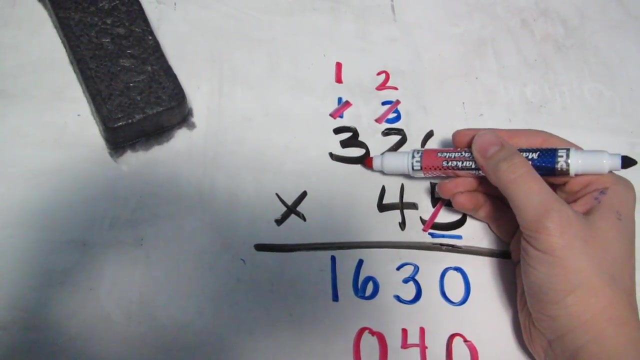 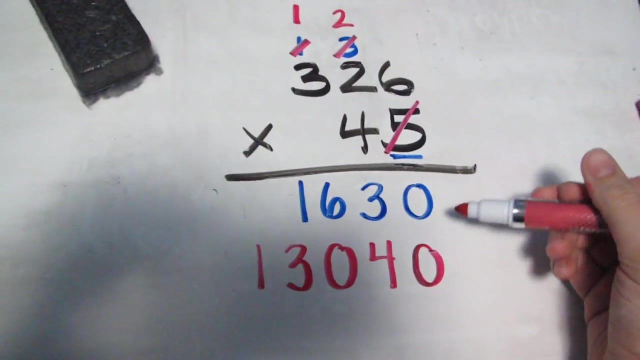 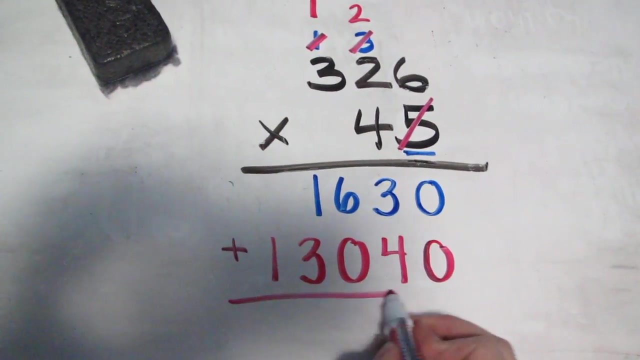 one, 4 times 6 is 24.. I'm going to do the same thing, 24.. Then I'm going to do 4 times 2, 8 plus 2, 8. So 4 times 6 is 10, 1, 0. And then 4 times 3, 12 plus 1 is 13.. See and notice again the whole time. I kept my numbers lined up nicely, So when I get to the adding part, all I have to do is put it together. 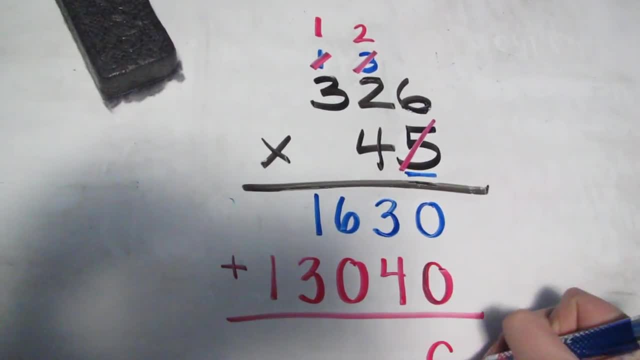 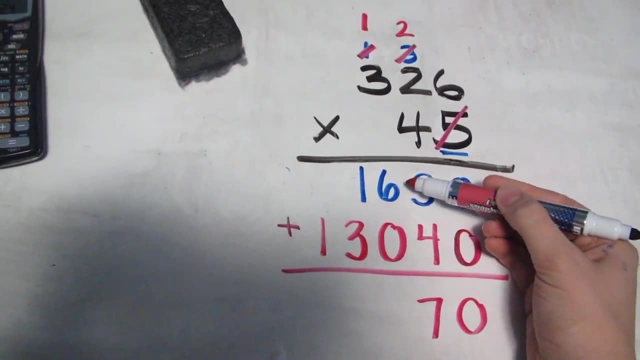 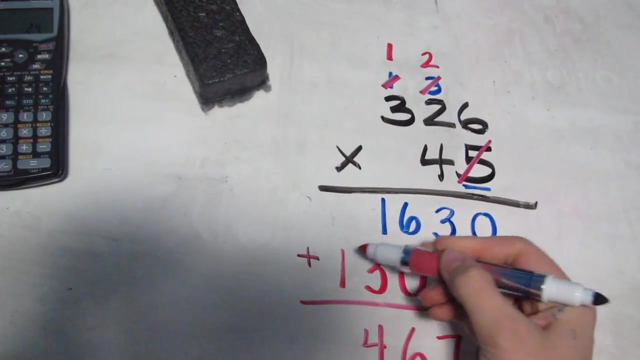 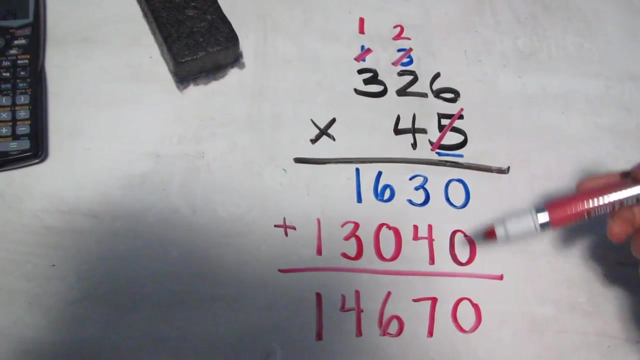 So 0 plus 0 is 0.. 3, 3, 3, 3 plus 4, 7.. 6 plus 0, 6.. 1 plus 3, 4.. And I bring down the 1, and I find out that 326 times 45 is 14,670.. 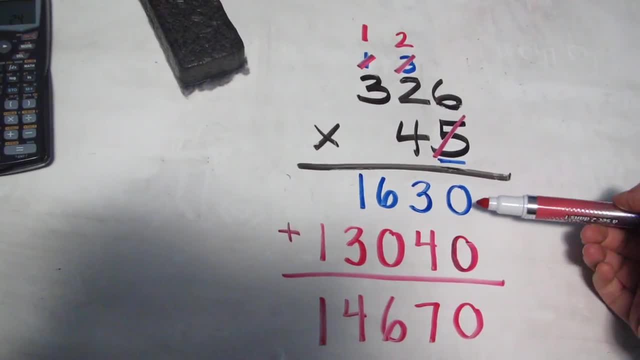 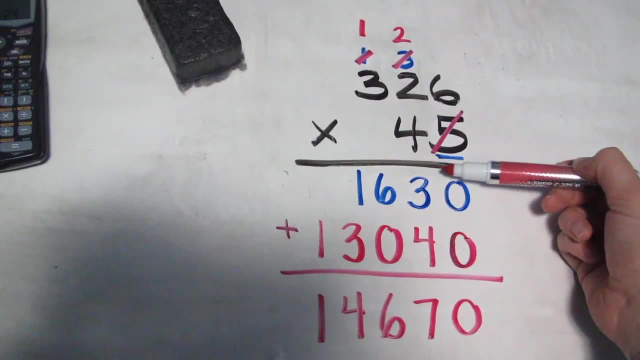 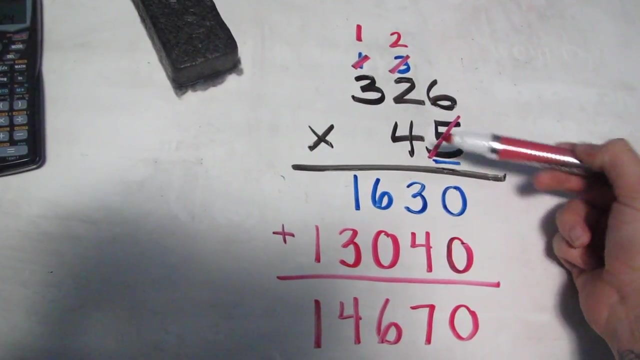 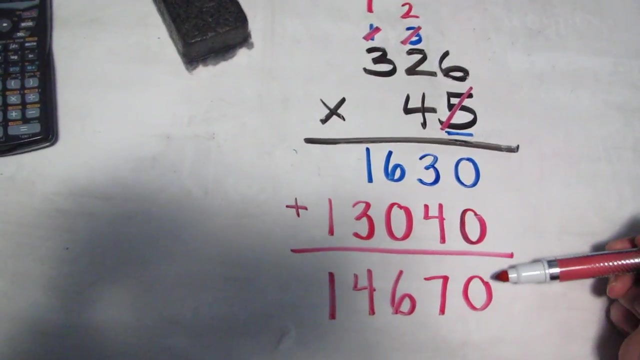 And so again, these two numbers mean that I multiplied everything in my 1's 1's place, that's this number and the things in my 10's place. So 326 times 5 is 1,630.. 326 times 40 is 13,040.. And I put those two together and I got my answer. 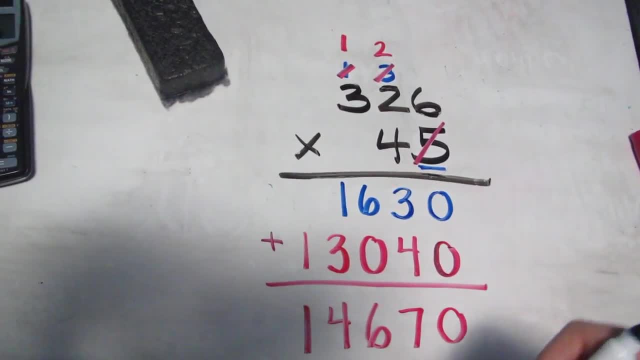 And that's how you do: 3-digit times a 2-digit number: 3, 3, 3, 3, 3 3.